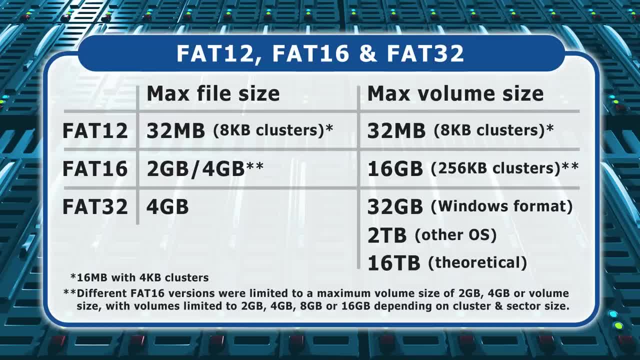 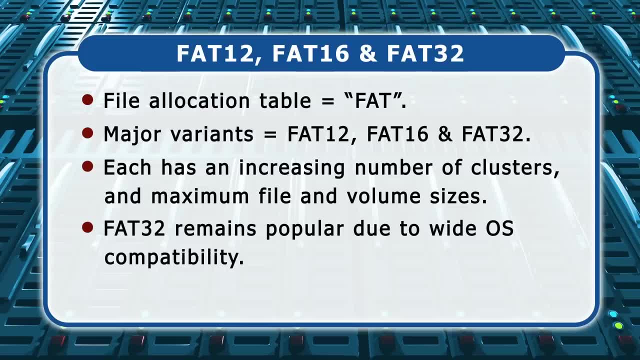 terabyte volumes when formatted with other operating systems and has an absolute maximum volume size of 16 terabytes. FAT32 remains a popular file system due to its high level of compatibility across operating systems and is still widely used to format USB flash drives, memory cards and some other. 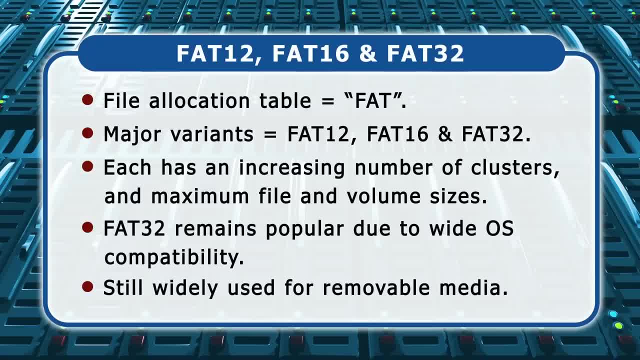 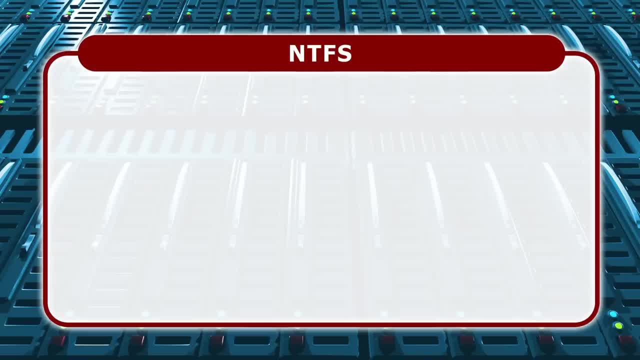 external storage devices. So how does FAT32 compare with other operating systems? Today, the most popular Windows file system is the New Technology File System, or NTFS. This was introduced in 1993 to overcome the limitations of FAT32 and has a file size limit. 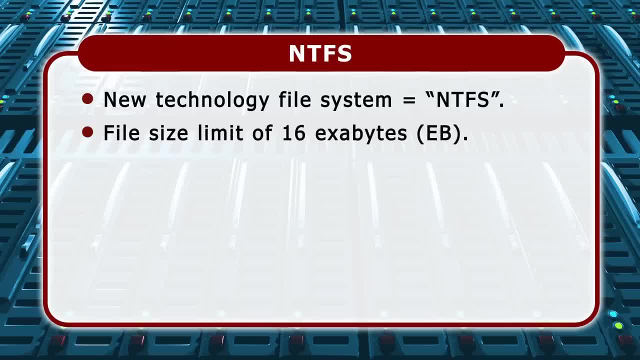 of 16 exabytes. An exabyte is one million terabytes, so in practice there's no file size constraint. NTFS is also a journaling file system, which means that it maintains a record of changes so it can recover following a system crash or power failure. 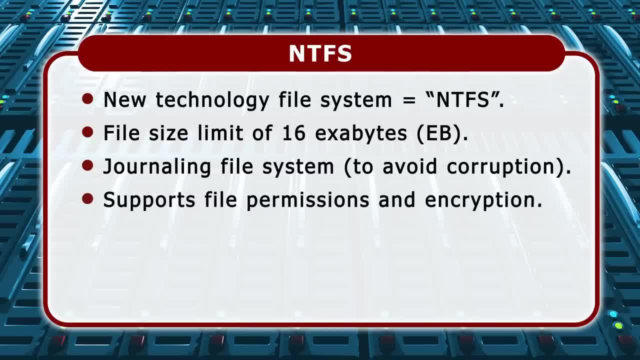 Unlike FAT32, NTFS also supports file permissions, for example, allowing a file to be flagged as read-only, as well as encryption and other features that make NTFS more suitable than FAT32 for use on a system drive. For these reasons, all modern versions of Windows must be installed. 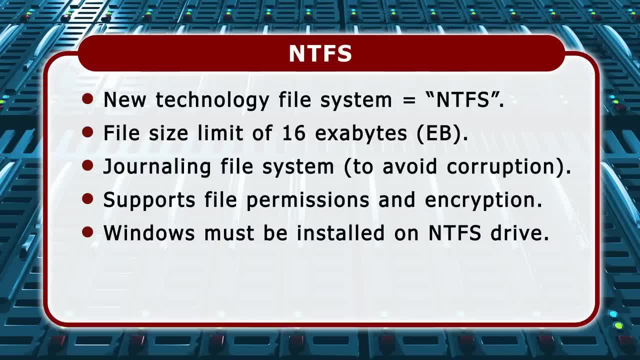 The only real downside of NTFS is a lack of compatibility with older versions of Windows and non-Windows operating systems. For example, by default NTFS volumes are read-only in macOS and in older Linux distros and may not be readable at all on other devices such as stand-alone media players. 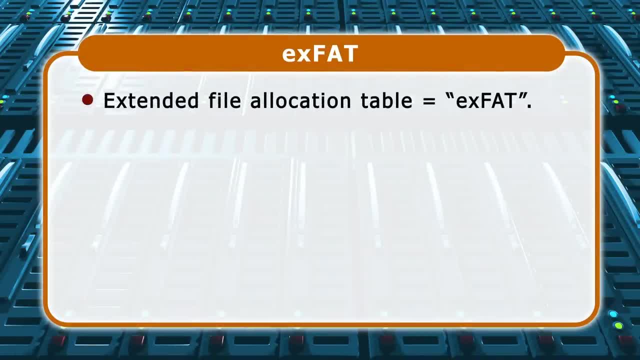 XFAT, or the Extended File Allocation Table, was introduced by Microsoft in 2006 as a file system optimized for high-capacity USB flash drives and memory cards. XFAT is less sophisticated than NTFS, but has significant benefits over FAT32.. Not least, the maximum file size is 16 exabytes, or effectively unlimited, which makes XFAT 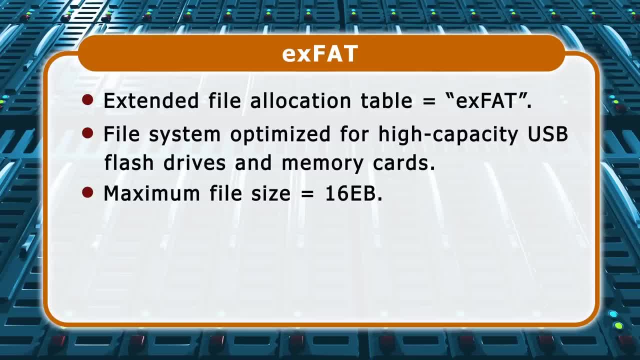 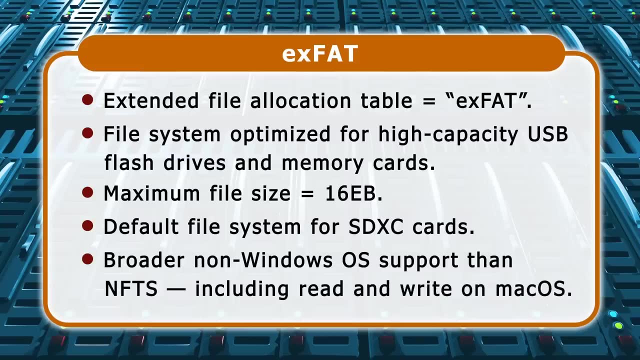 the best choice for formatting memory cards for recording video. For this reason, XFAT has been adopted by the SD Card Association as the default file system for SDXC memory cards. In terms of compatibility, XFAT enjoys wider non-Windows support than NTFS with read-and-write. 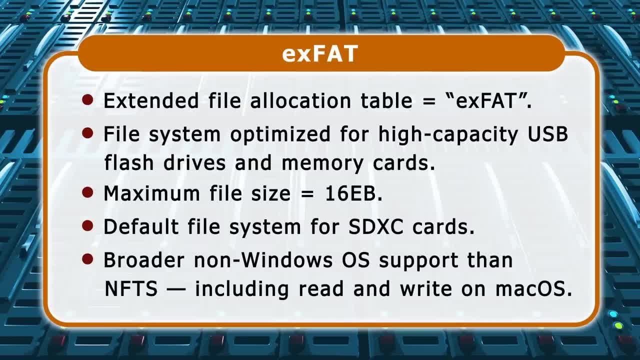 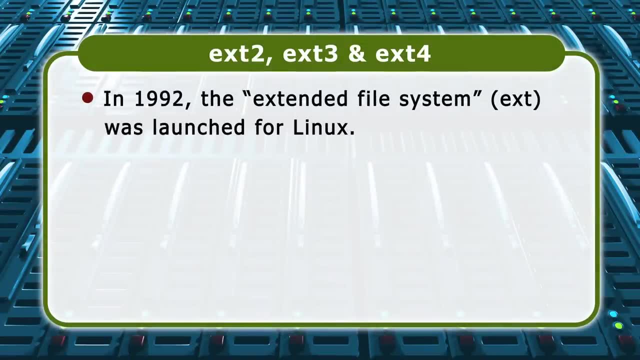 support on Macs and recent versions of Android. This said, many Linux systems require extra drivers to be installed to access XFAT devices. Talking of Linux, in 1992 the Extended File System, or EXT, was launched specifically for this operating system. 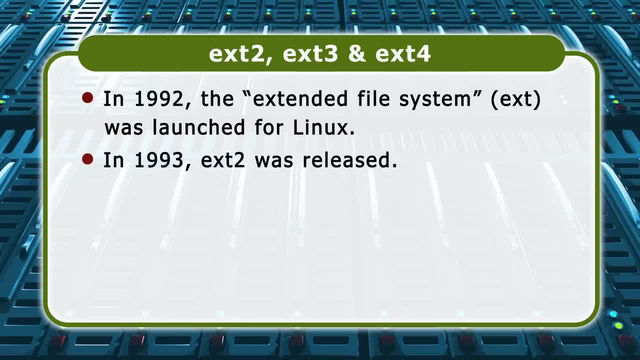 In 1993, an update called Extended File System 2, or EXT2, was then released and was for many years the default file system in many Linux distros. By 2001,, EXT2 was upgraded to EXT3, which introduced journaling to protect against corruption. 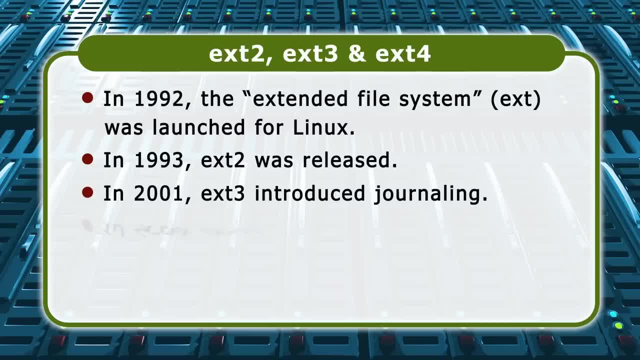 in the event of crashes or crashes In 2008,. we then saw the release of EXT4,, which is the most modern dedicated Linux file system. EXT4 has a maximum file size of 16 terabytes and a maximum volume size of 1 exabyte. 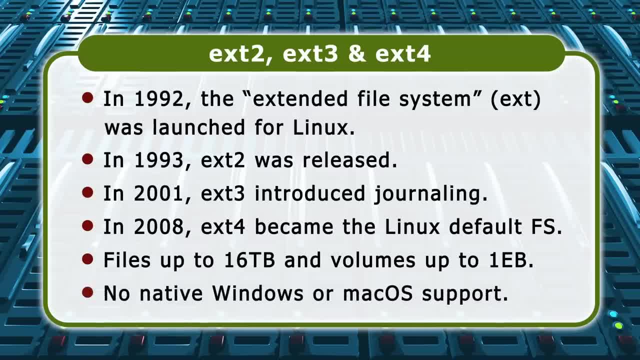 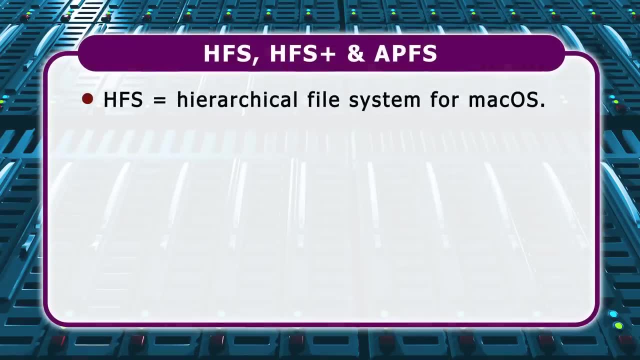 However, as you may anticipate, neither Windows or Mac OS offer native EXT2, EXT3 or EXT4 support. HFS, or the Hierarchical File System, was introduced by Apple in 1985 for use in Mac OS. It offers a maximum file size of 2 gigabytes and a maximum volume size of 2 terabytes, and 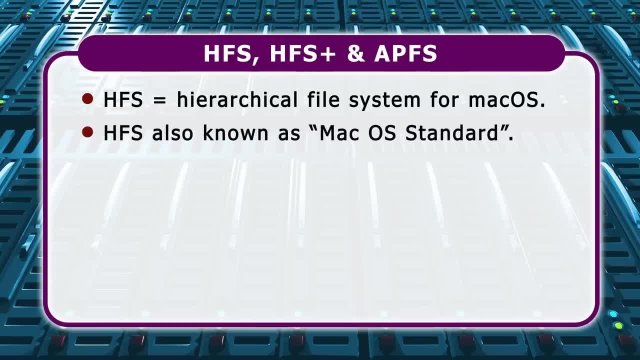 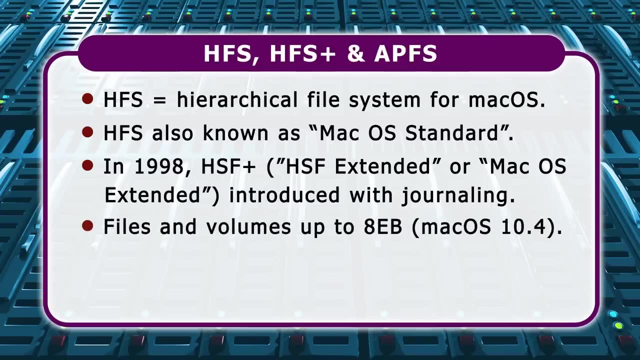 is also known as Mac OS Standard. In 1998, HFS was upgraded to a new version called HFS Plus or HFS Extended, otherwise known as Mac OS Extended. This added journaling and has a maximum file size and volume size of 8 exabytes. when using 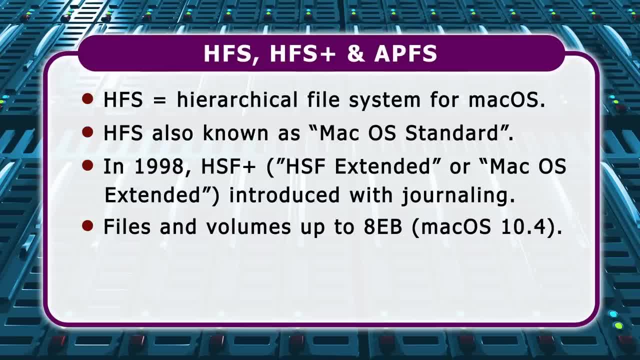 Mac OS 10.4 or above. In 2017, Apple introduced a new file system called APFS or the Apple File System, which is optimized for SSDs and other solid-state media. Hardly surprisingly, HFS, HFS Plus and APFS are not natively supported by Windows or other. 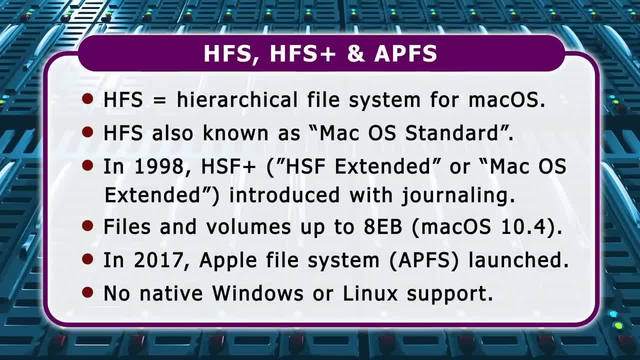 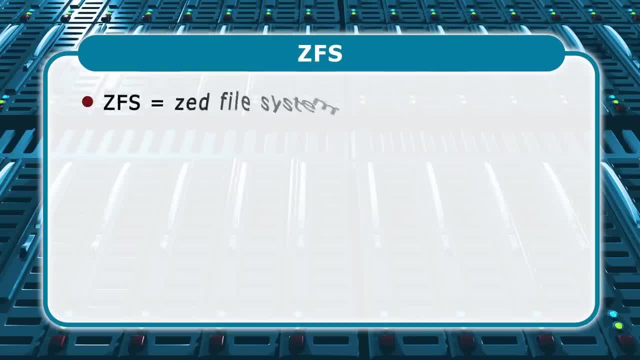 non-Apple operating systems. Finally, I thought I'd mention ZFS, or the Zed File System, Initially released in 2006,. this was created by Sun Microsystems, but since 2013 has been developed by the OpenZFS project. 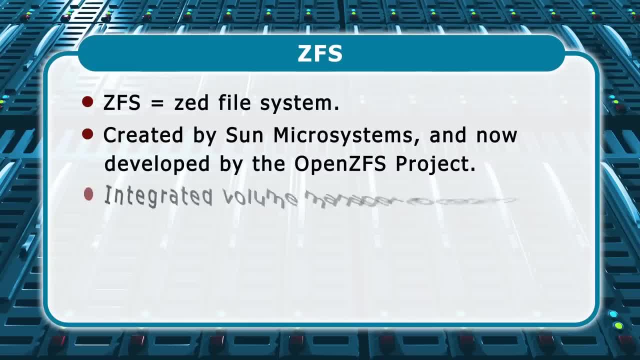 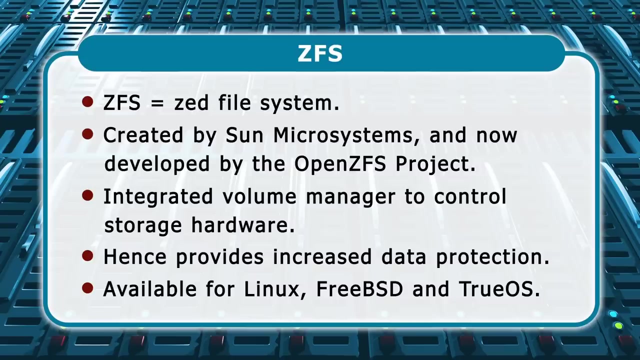 ZFS differs from other file systems because it integrates a volume manager to control the storage hardware attached to a computer. By integrating physical drive management with file system functionality, ZFS provides increased protection against data loss or corruption. ZFS is currently available for Linux, FreeBSD and TrueOS and in the future may be ported. 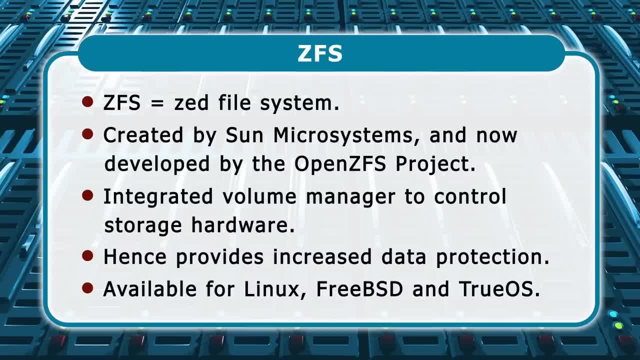 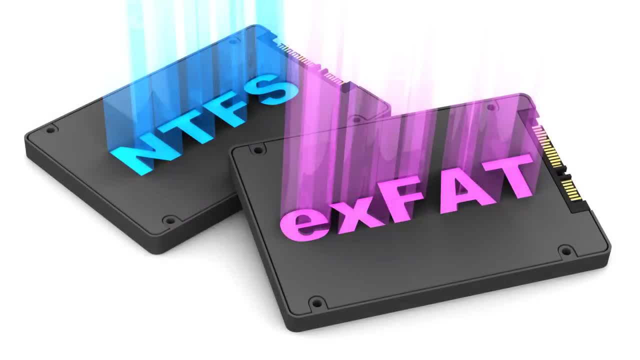 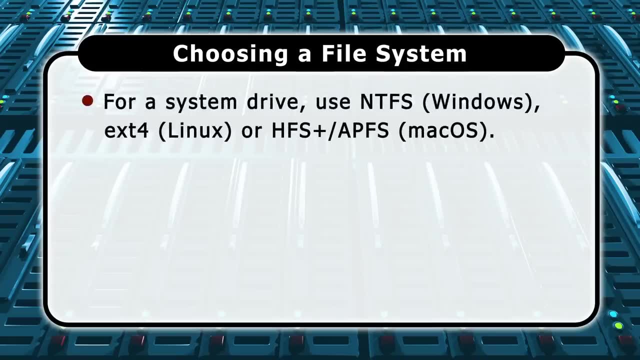 to Windows and MacOS. So which file system should you choose? 1. Well, for your system drive, you should or must choose the file system for your chosen operating system, which means NTFS for Windows, EXT4 for a Linux distro, or HFS Plus or APFS. 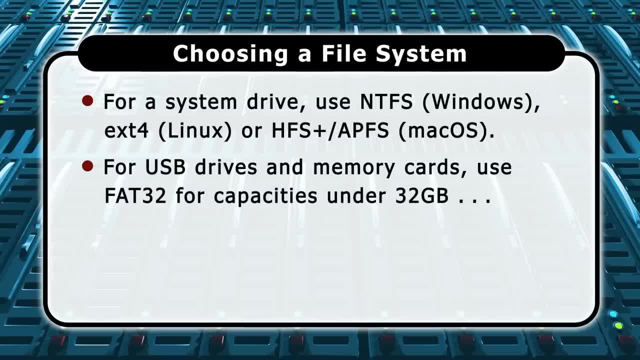 on a Mac For USB drives and flash memory cards. FAT32 remains the best choice for devices below 32GB in capacity in order to maximize compatibility across platforms. 2. Well, XFAT is the best choice for a flash drive or memory cards of 32GB capacity or 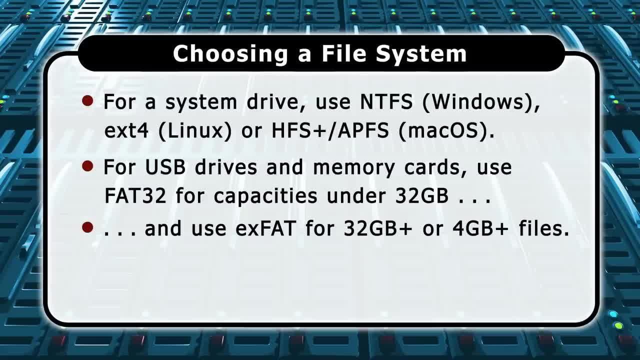 more, or when you need to store files greater than 4GB in size For external hard drives or SSDs. NTFS is the best choice for anybody who is entirely or primarily Windows-based, while XFAT is probably the best choice for anybody who regularly. 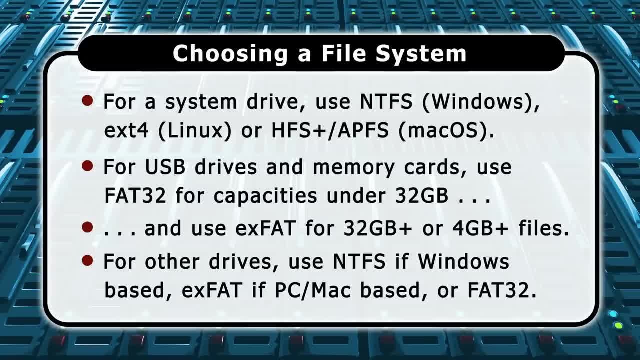 shares files between a PC and a Mac. 3. For file size and volume size limitations, FAT32 also remains an option for external drives that need to be accessed across a wide range of Windows, Mac and Linux systems. 4. What is a single board computer? 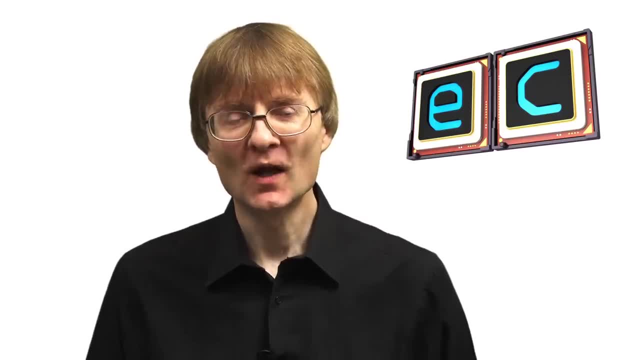 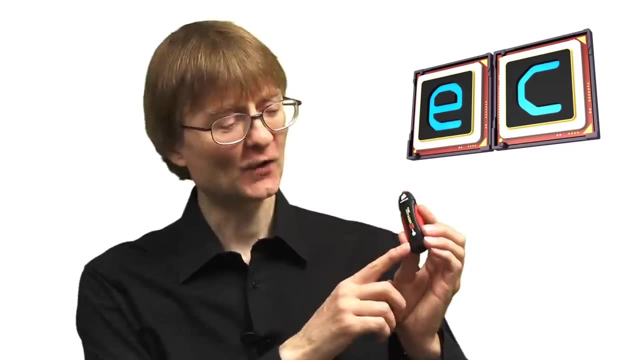 Several years ago I was making an Explaining Computers video about a single board computer and I had to download an operating system image. I did so. I downloaded it to a flash drive. I had to decompress that file so I could use it on the single board computer.